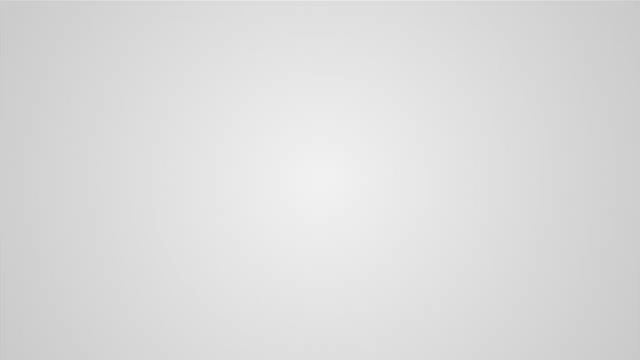 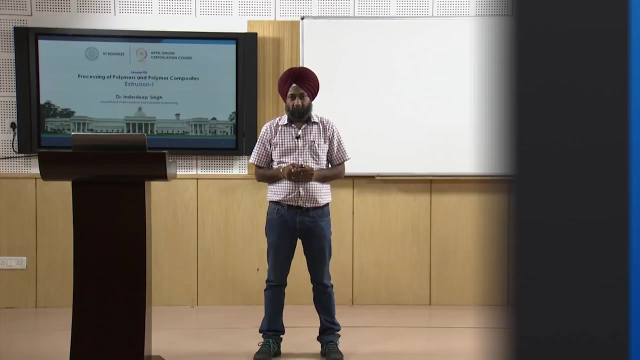 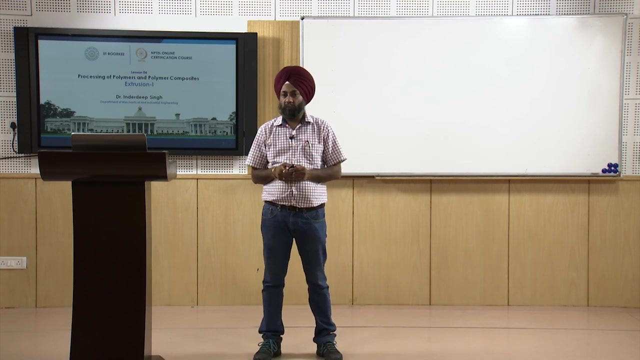 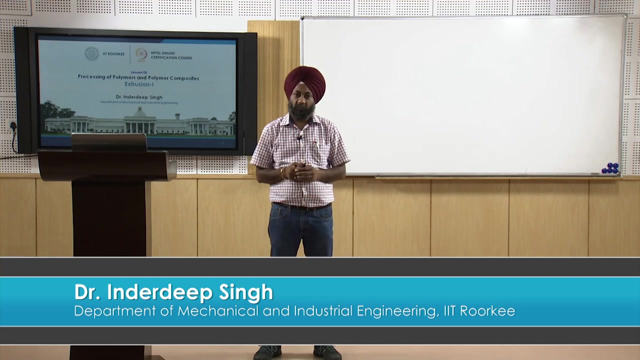 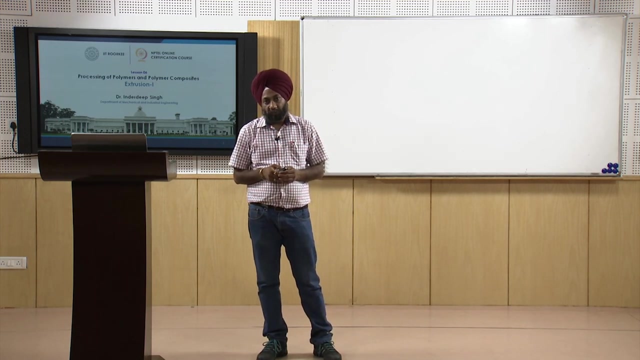 Namaskar friends, welcome to this lecture six in our course on processing of polymers and polymer composites. if you remember, in the last sessions we have discussed the basic properties of the polymers. we have also started our discussion on the various processing techniques for polymers. we have already covered two processes, that is, casting, as well as thermo forming. 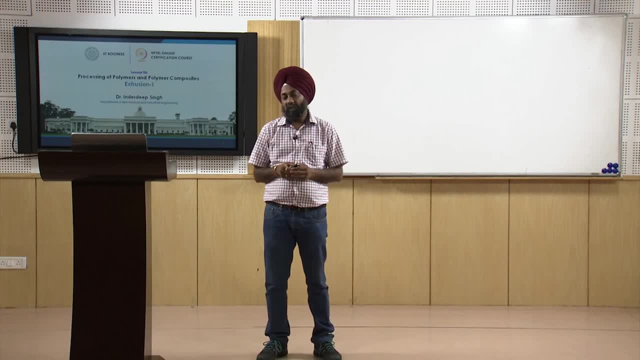 in casting. we have seen that it is a most simplistic process and we can use both thermosets and thermoplastics majorly used for thermosets, and we can give shape to the polymer using a mold cavity or a metallic mold in case of thermo forming. if you remember, it is used majorly for thermoplastic sheets very thin. 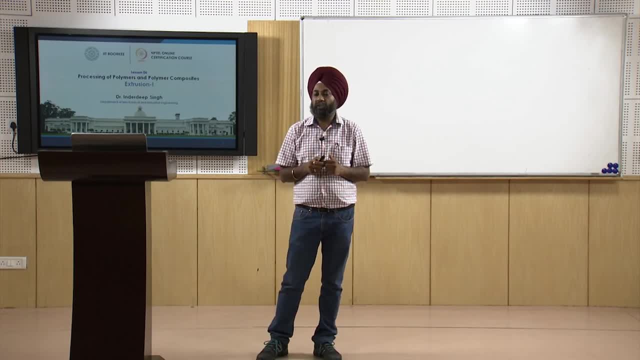 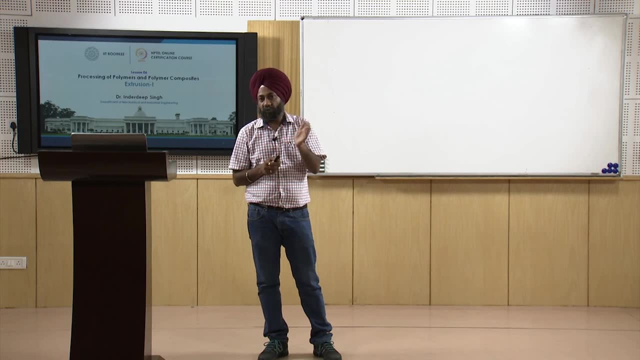 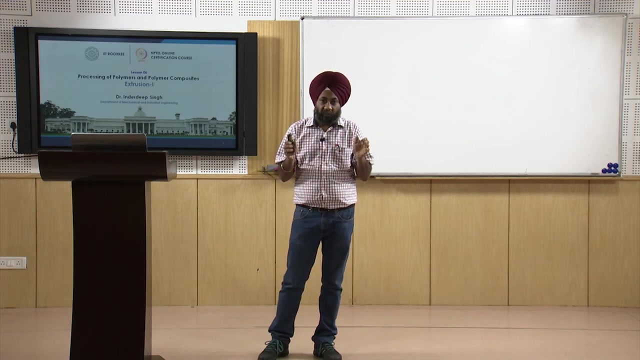 sheets and we can give desired shape to these sheets with the help of three types of pressure. we have seen vacuum thermo forming, we have seen pressure thermo forming and we have seen matched die type of thermo forming process. So if you, if you see that we have already tried to understand two important processes that are used for polymers and in 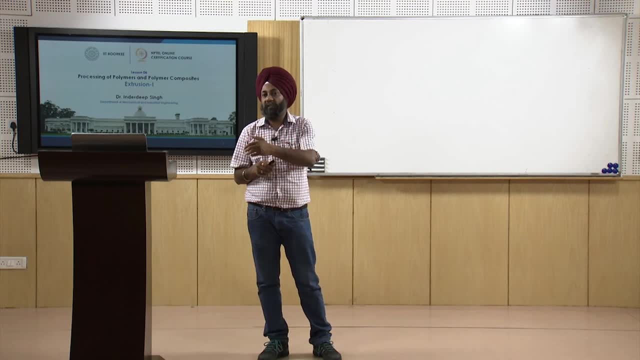 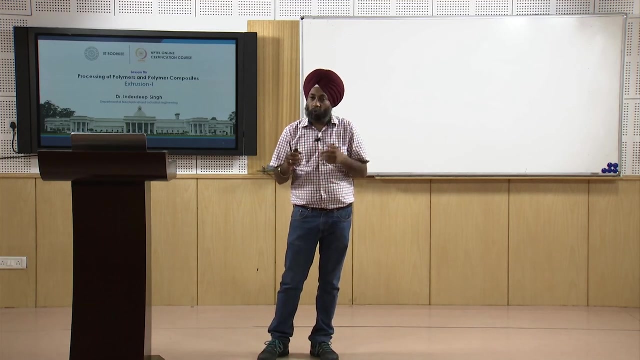 both the processes, plus in the processes that we are going to cover in our subsequent lecture. you will try, you will understand that there are three components- again i am emphasizing that- heating, forming and cooling- that are common, so that we are going to see today. also, if you see the topic that we are going to cover today, it is extrusion, now extrusion. 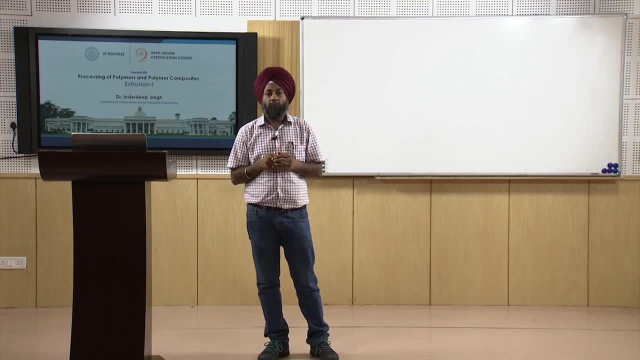 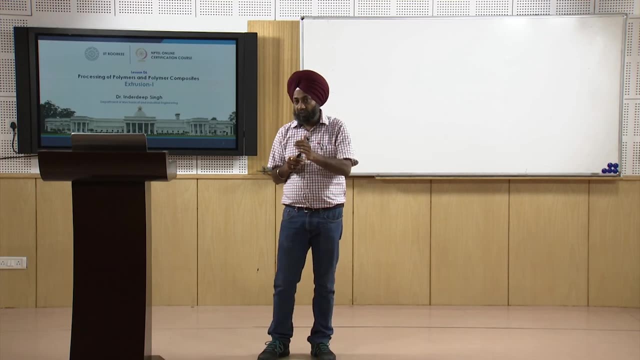 is a most widely used process for processing of polymers and we will see that how the plastics are processed using extrusion, what is the process, what are the various parts of extrusion of machine. we will try to understand that. what are the important control parameters? what are the different types of products that can? 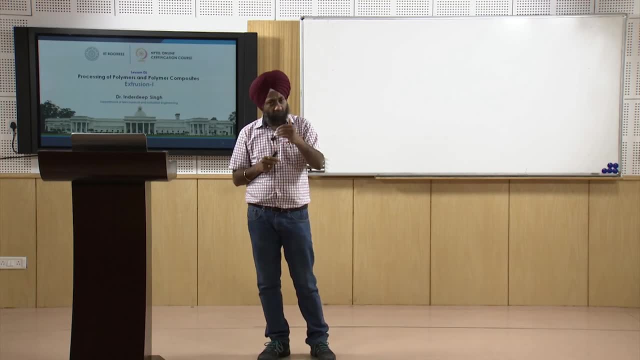 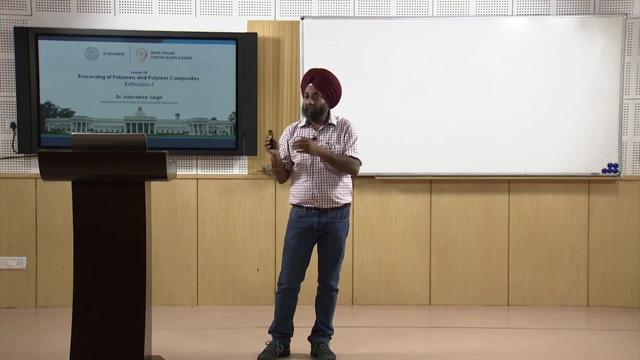 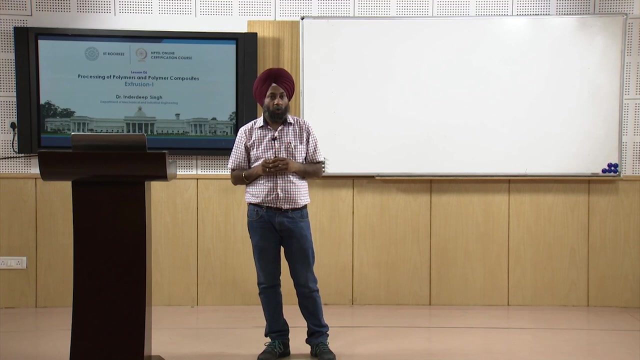 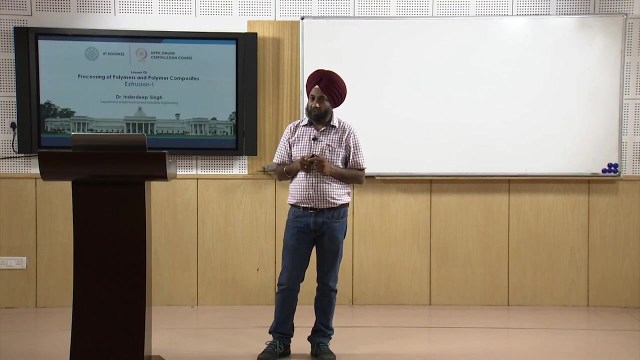 be made, and then we can always ah understand the things better if we have a video which represents the process. So today we will see a very small video ah give a complete description of the whole process, that how the process operates and finally makes a product out of a plastic. so let us start our discussion on extrusion. 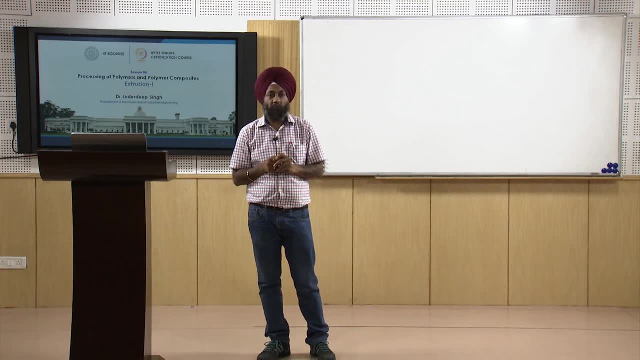 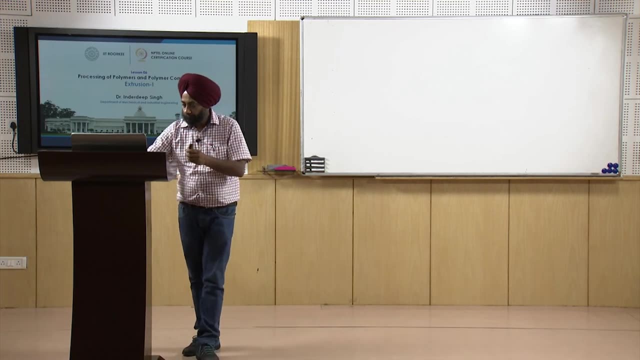 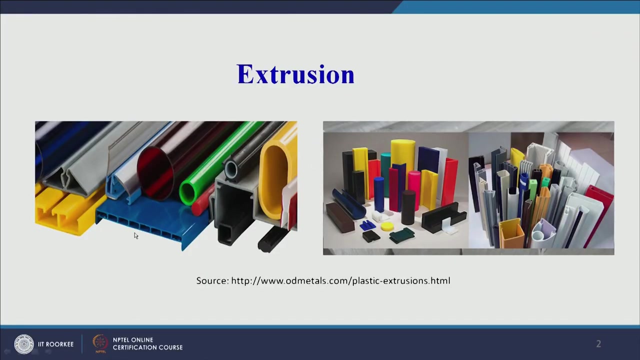 and we will cover whatever i have listed down in the beginning of the session, that all these things will be covered in todays session. so let us start our discussion. on your screen you can see that different types of products with different colors are processed for plastics. so if you see yellow color, blue color and first let us start first. 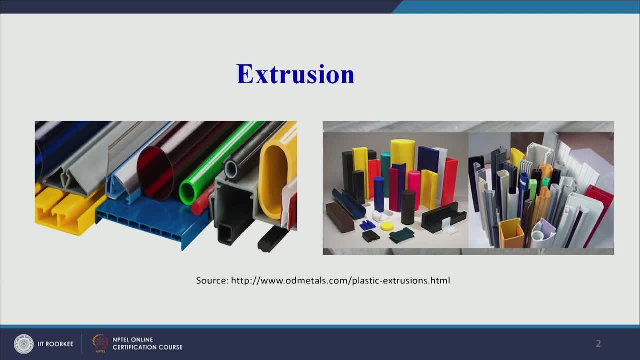 i want to grab your attention towards the products that are made. then we will go to the technical aspects of the products. if you see, different colors products can be made. that is one versatility of the process, that it is not color specific. any color can be made. so if you can appreciate the colors that are made, then you can understand the process and 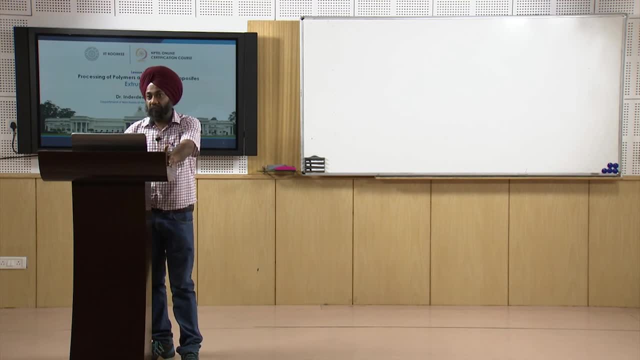 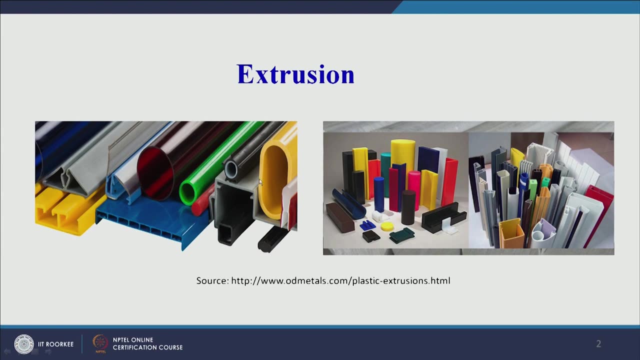 you can appreciate that. then you can see the shapes, which is a technical parameter. so if you see the shapes, there are circular cross sections. there are maybe, ah, different types of cross sections. square cross sections are there, oval type of cross section is there. then we can see, ah, special design, a honeycomb type of cross section is there. so, depending. 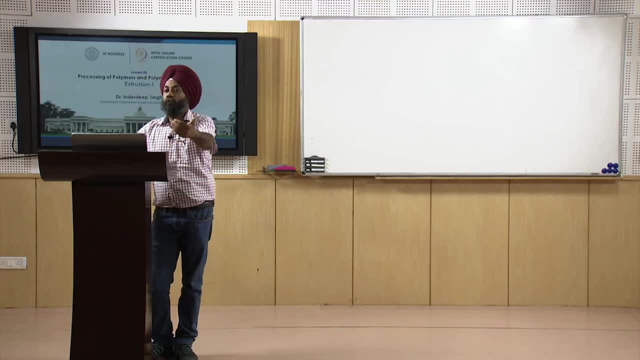 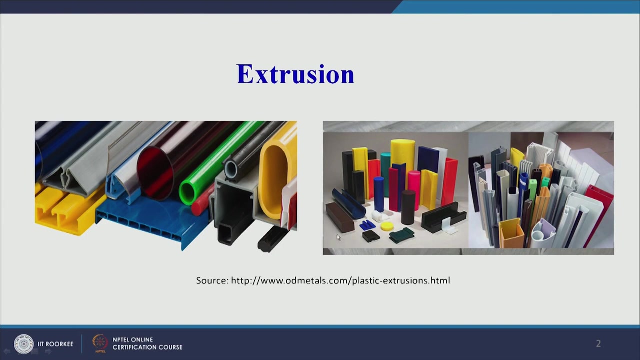 upon the cross section. we can make a use of the extrusion process and we can make a product. so on this side also, the other view of the product, also the other view of these products, you can see there is a angle section here. there is a solid cylindrical cross section. the solid cylinder has been made. there is a rectangular. 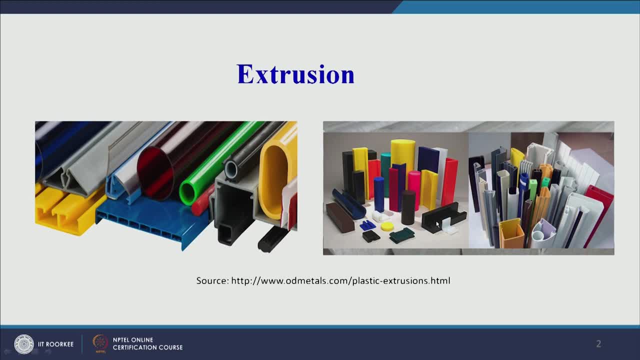 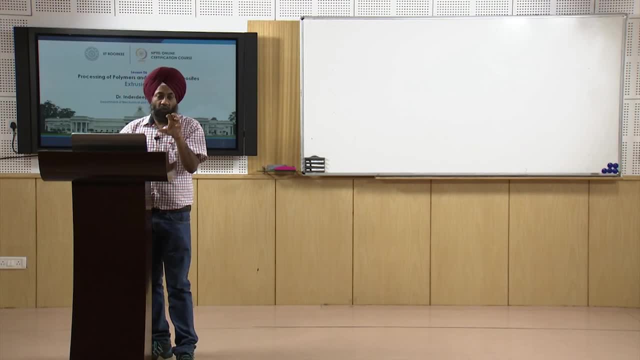 type of cross section and there is a complicated cross section also. so extrusion process is a versatile process and everything depends upon the die, or the or the heart of the extrusion machine, that is, the die. now, depending upon the product, we have to design the die and 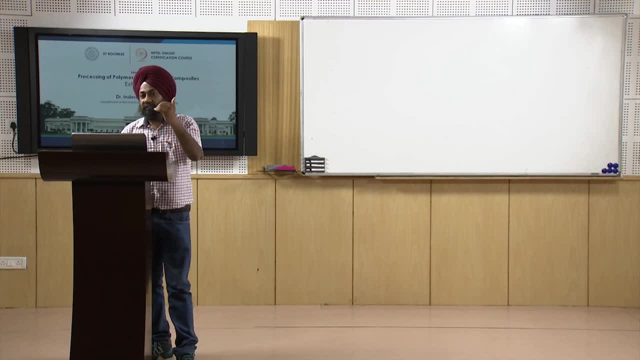 the digitales. the die will give us the desired shift the things, as i have already told, we have to heat the plastic material. once it is hot, it will post through the die. depending upon the shape of the die, it will take the desired shape. finally, the product, that is. 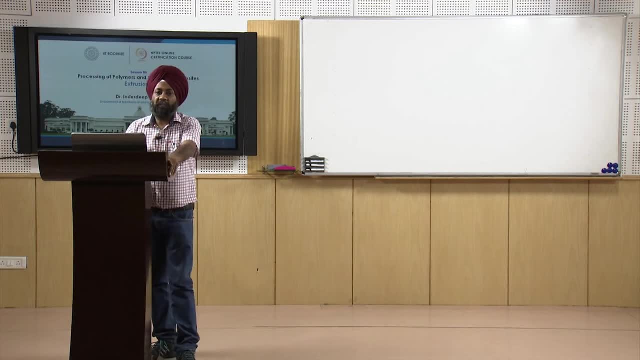 coming out of the die, we will call that product and, finally, our product will be ready and, depending upon the length that we require, we will cut the product into desired cross sections or not. the desired cross sections section: the desired length across the cross section, so that we get the product in the 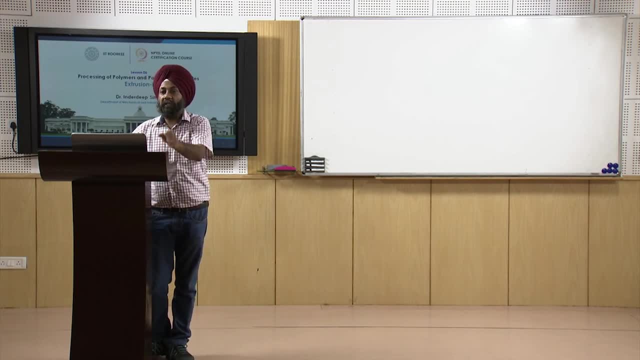 video. it will be very, very clear so you can see the different types of products that we can make using the extrusion process. just to explain you the importance of this process, i can just share with you that the gardeners pipe that we use in for watering the plants. 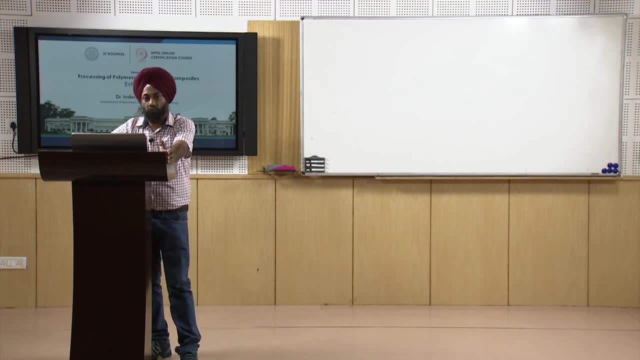 or sometimes for washing our cars. also, the plastic pipe that we use that is made by the extrusion process, so that you can appreciate, relate to the process that what is extrusion. so let us start our discussion with the extrusion process. extrusion is a high volume manufacturing. 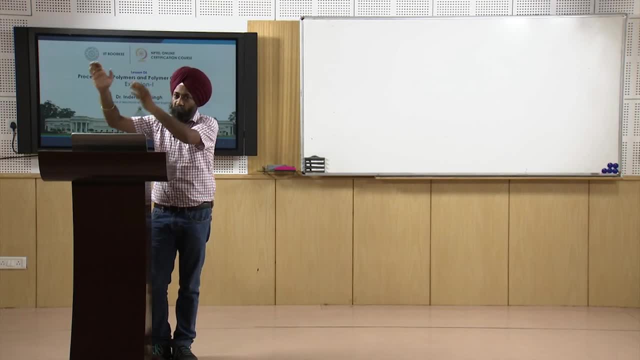 process. so you can see it is a continuous process. once you feed your raw material, which is available in the form of pellets, so these pellets will be melted and then they will be forced through the die and continuously the production can be there. so if you see, you have long gardeners pipe, long hose pipes. 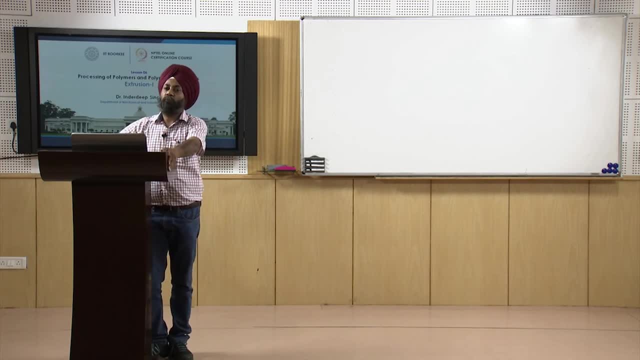 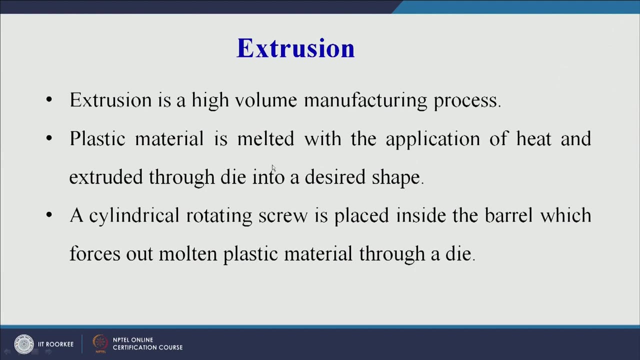 so that that means that they have been produced through a continuous process of manufacturing. so extrusion is a high volume, continuous manufacturing process. plastic material is melted with the application of heat and extruded through the die into the desired shape. i have already emphasized this point: that heat for your heat, your deformation, ah, in the form of a die and 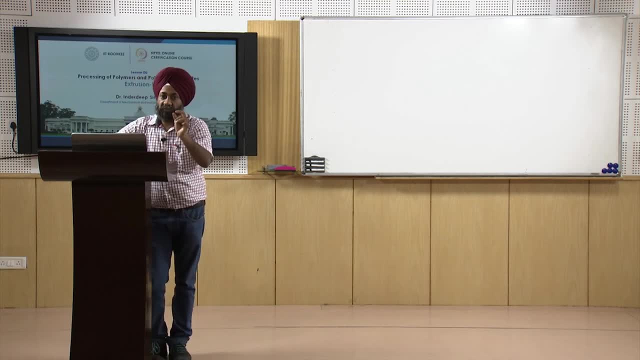 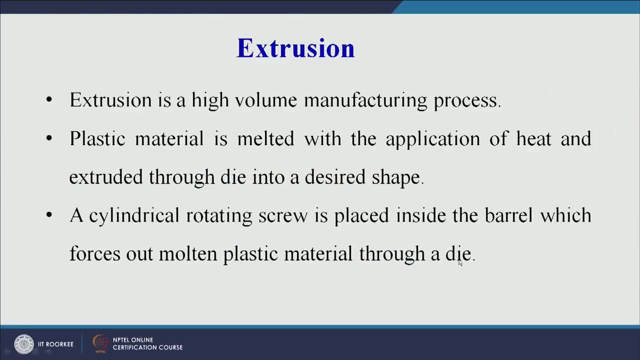 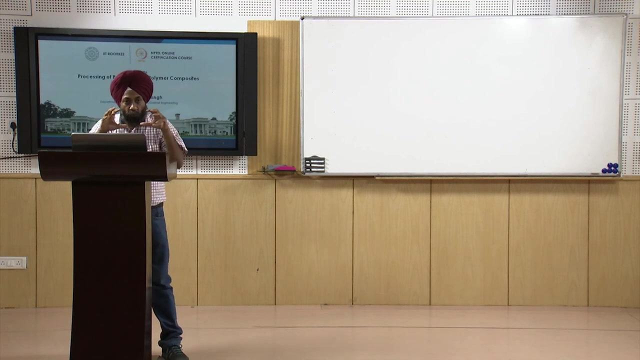 finally, the cooling are the basic principle, are the basic steps involved in the extrusion process. a cylindrical rotating screw is placed inside the barrel which forces out molten plastic material through the die. now something has to be there which will push the material through the die so that work, that is, pushing the material through the die, is achieved by 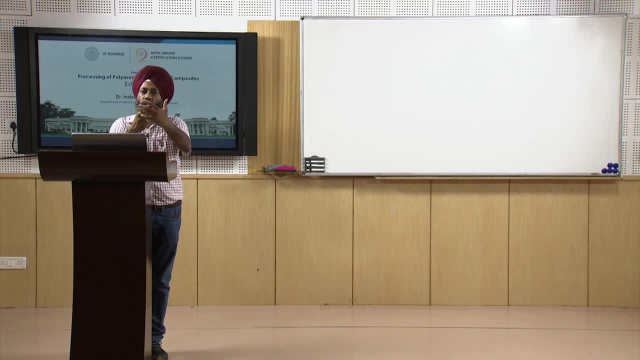 the barrel. you can try to understand this with the help of a surgical syringe in the syringe. the syringe is the syringe which is used to push the material through the die syringe. what is done? first you pull the medicine inside the syringe and then you apply the 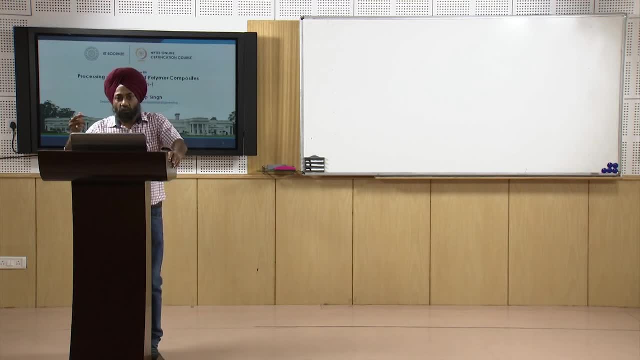 pressure and inject the medicine into the human body or into the animals body. so the same principle, you can correlate that medicine with the plastic. now you have a plastic inside a barrel. you have to push it so that it comes out, so die in this case, can be the needle. 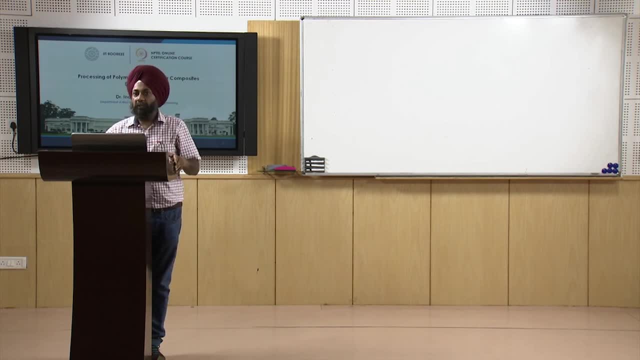 through which the medicine comes out. so that is the principle, but here that piston cylinder arrangement. in place of the piston cylinder arrangement, many a times we use a screw and barrel arrangement through which we have the plastic. we push that plastic with the help of a screw and it is forced through the die into the mold cavity. in this case it will. 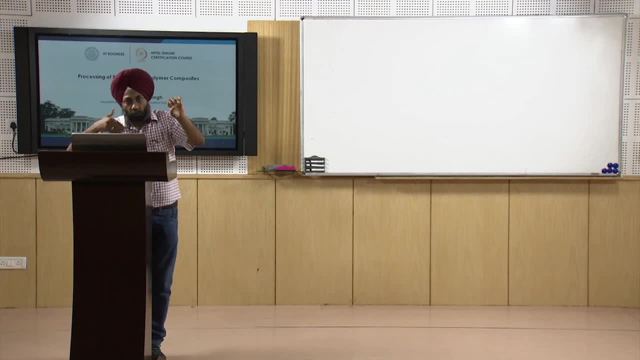 not be a mold cavity, it will be a die. so you will push the molten plastic through the die and die will be the exact replica of the final product that we want to make now, as i have shown in the previous slide. different types of die are there different types of die will. 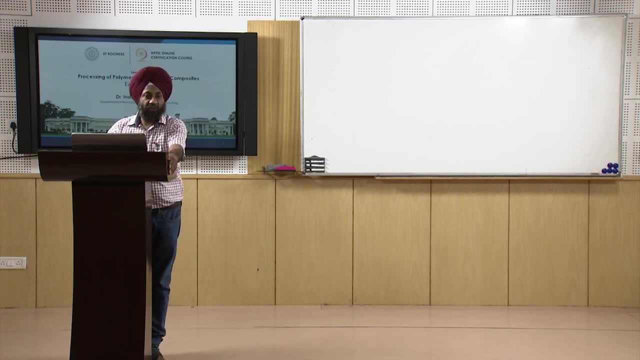 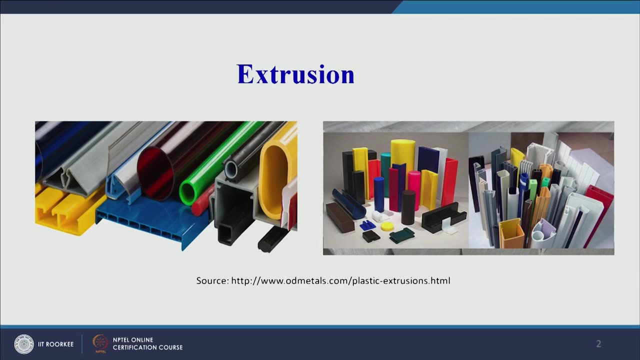 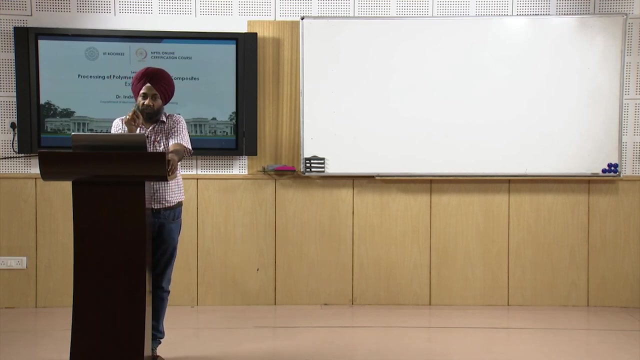 be there different types of die? are there different types of die? are there different types of products can be made on your screen, you can see so these products the shape of this product will depend upon. you can very easily now answer this question: the shape of this product will depend upon the shape of your die. now, if it is a circular die, you 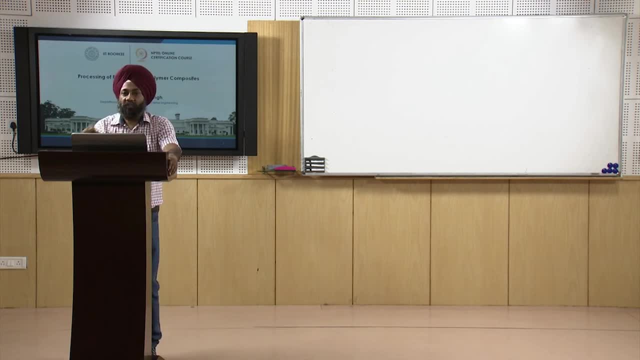 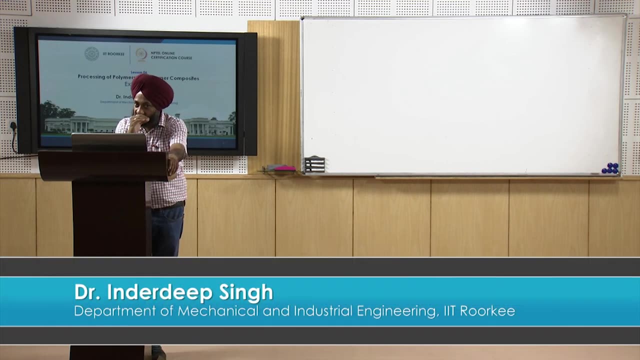 will get a circular product. if you have a square die, you will get a square product. now, depending upon the shape of the die, you will get your product. so that is. these are three basic steps, that is, heating of the plastic, pushing of the plastic through the die and 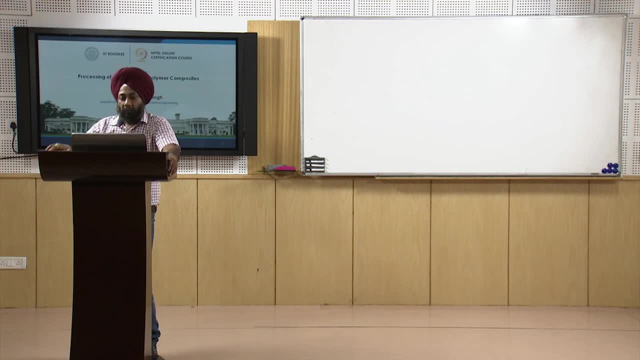 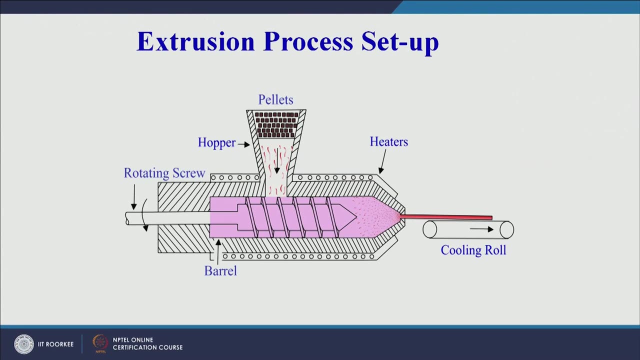 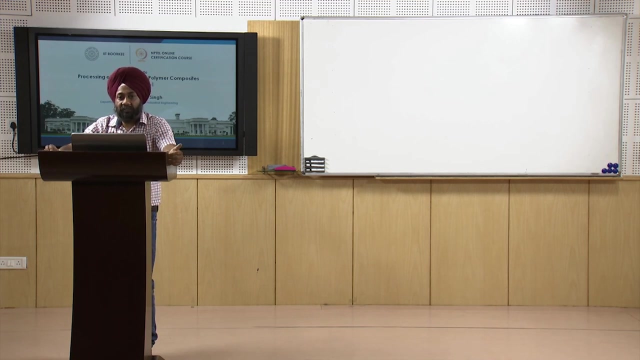 cooling of the product when it comes out of the die. on your screen now you can see a very simplistic representation of the extrusion process. there can be so many other components in the extrusion machine, but we are trying to understand the very basic mechanism of the extrusion process. so if here you can see there are for any process. 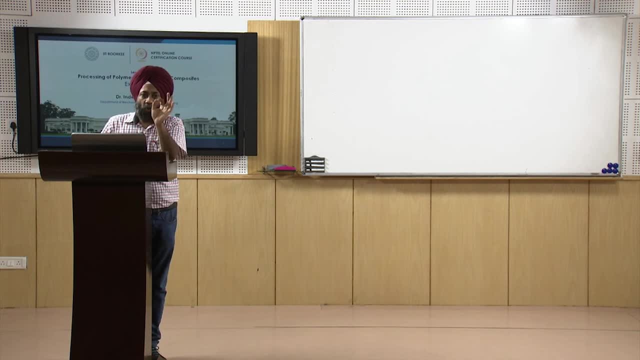 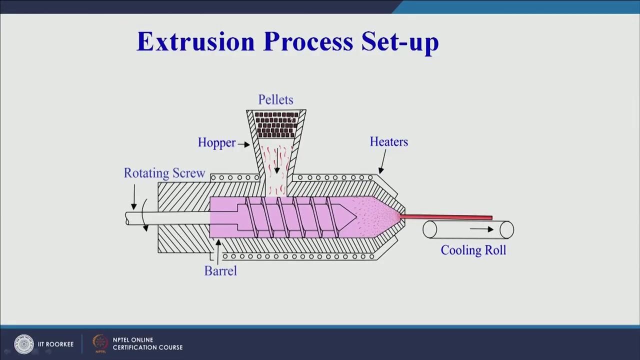 there are three things those are important: first is the raw material, second is the process mechanism and third is the product. so here let us start from the raw material. so raw material in case of for extrusion process are the pellets on your screen. we have this setup. these are black portion particles. are the pellets. so usually we get for thermo plastics. 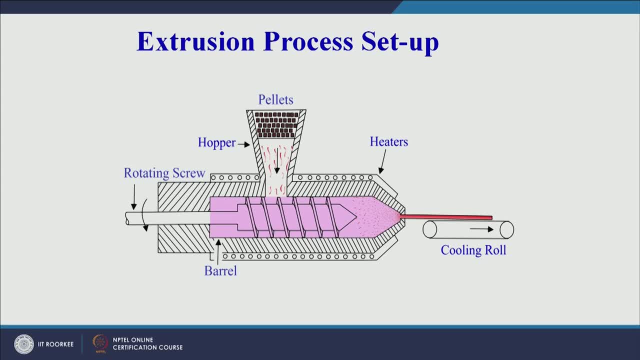 we get spherical pellets and those pellets act as the raw material for the process. these pellets move through this hopper into the barrel. this is a barrel portion. i am highlighting that barrel portion. so that is the barrel, and there we have this rotating screw. the rotating screw has also a specific design that we will cover towards the end of today's. 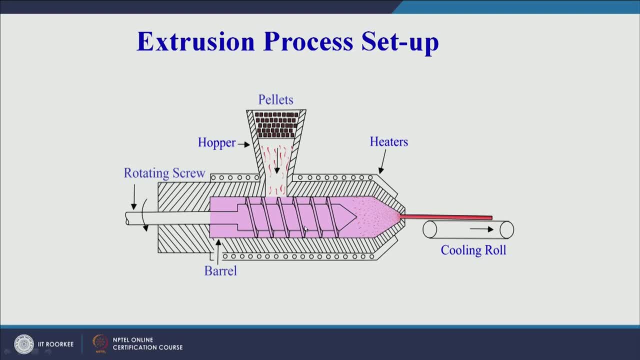 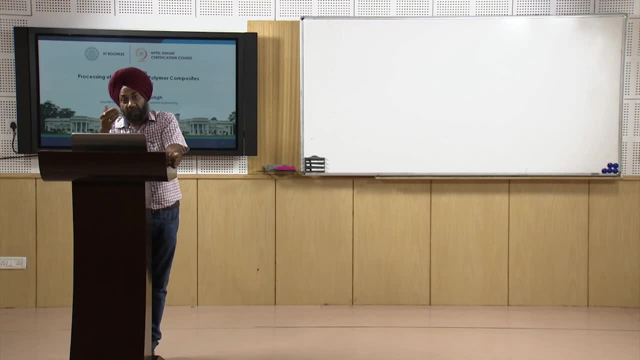 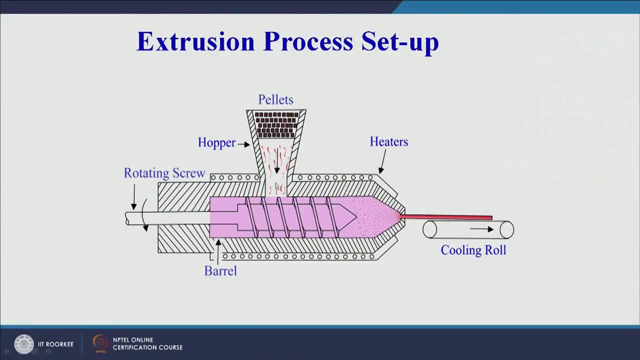 session. so there is a screw, there is a barrel, there are pellets that are coming down. now pellets are solid, spherical particles. we have to melt them and for melting we require heat, and for heating we require heaters. So on your screen you can see all around the periphery of the barrel. we have heating arrangement. 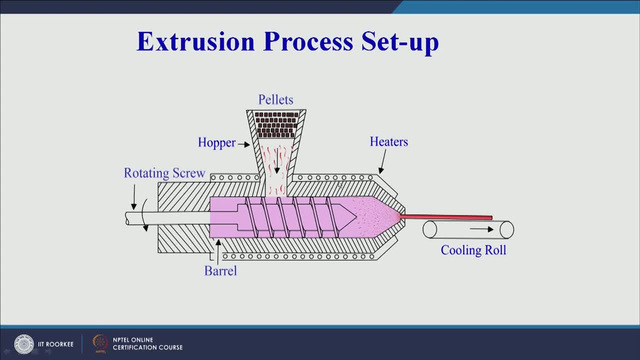 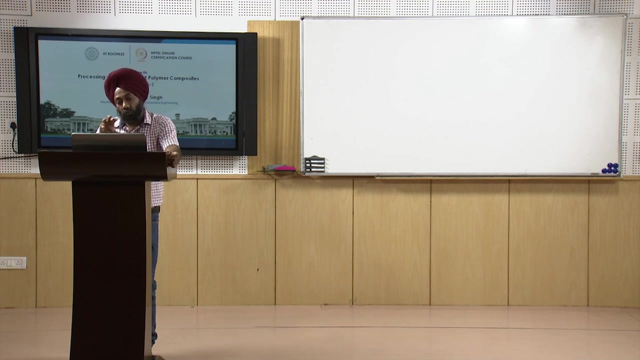 These square dots- sorry, these circular dots- represent the heaters. So these are the coils, or the heating coils. These circular coils here also represent the heaters. So you have heaters all around the barrel. So these heaters will heat the polymer pellets and will melt them. and once you melt them, 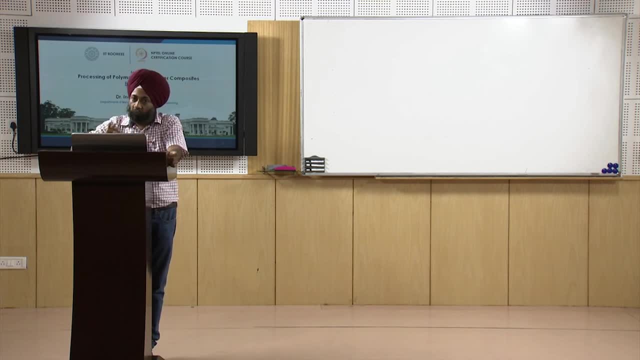 next stage is you have to push them through the die and then your product will be formed. So here we have the die arrangement, This is the place where we will have the die, and then this red colour portion is the final product that is coming out. 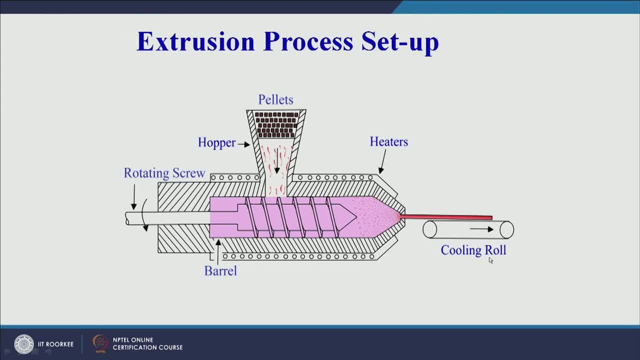 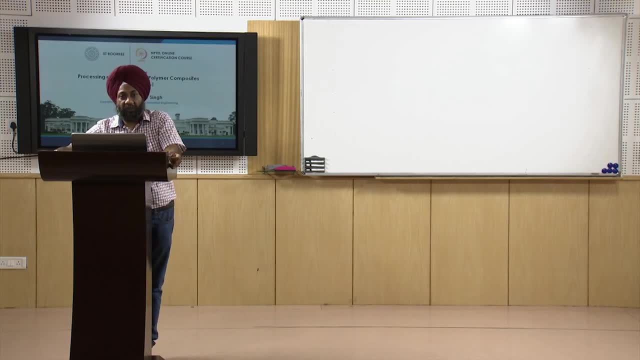 Now this product is rolling on a cooling roll And we can have. we will see in our subsequent slides when we will try to study step by step that how the process operates. We will see that the cooling can be water cooling, it can be air cooling. but right now 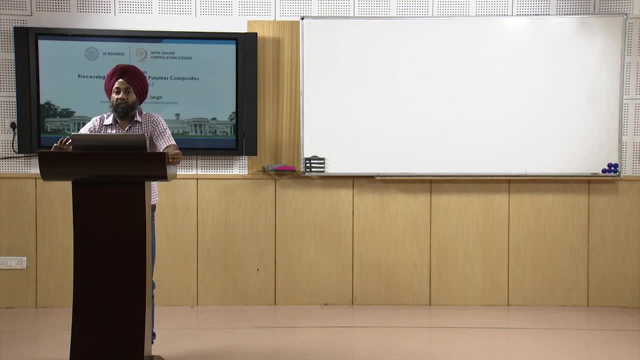 with the help of this diagram, we are trying to understand the how the extrusion process works in case of plastics. All of you may have studied extrusion of metals, So there are different variants of extrusion of metals, but here, in case of plastics, there 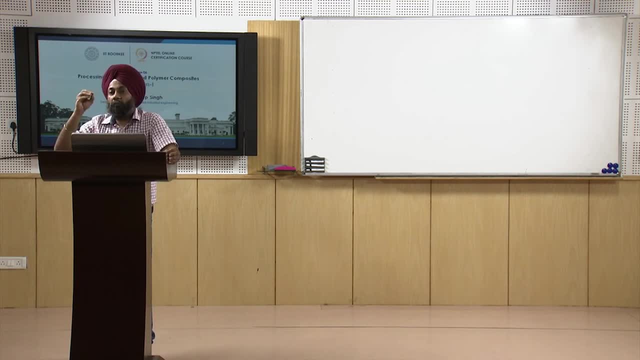 is a slight modification as compared to how the raw material is fed into the machine, How the product comes out from the setup. All these are the different things as compared to the extrusion of metals. So here you can see. once again. I am repeating, just may be 3 or 4 sentences. 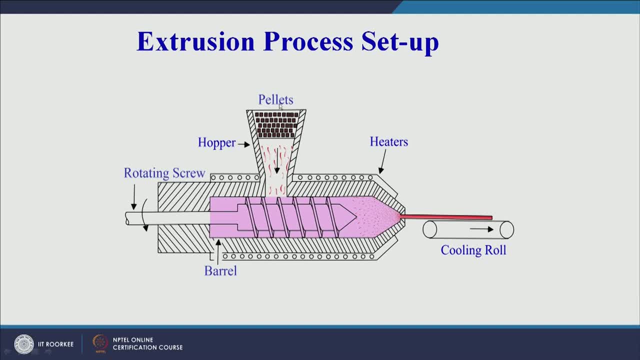 We have polymer pellets, thermoplastic pellets, here. These pellets are fed into the barrel. There is a rotating screw inside the barrel. The barrel is heated with the help of heaters. all around the periphery of the barrel barrel the rotating screw rotates and it pushes the molten plastic through the die a for onto. 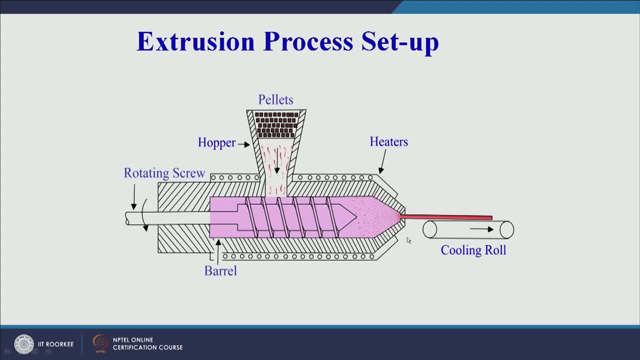 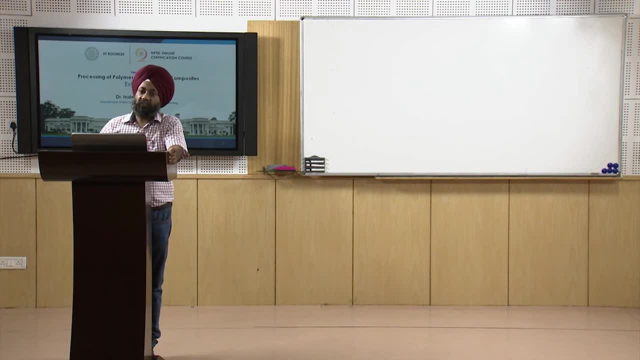 the cooling roll and your final product comes out from the die. so that is the basic working principle of the extrusion process. now let us read whatever i have said so that we are able to remember that what is extrusion process actually now? plastic material in the form. 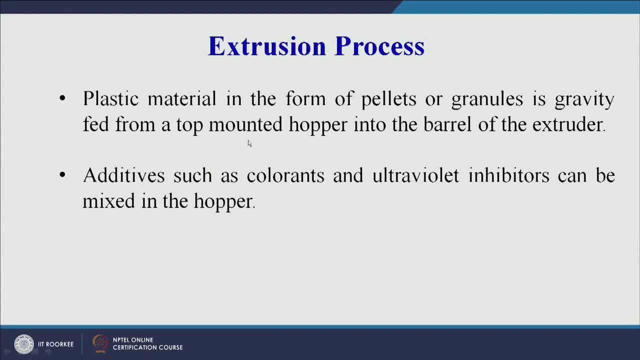 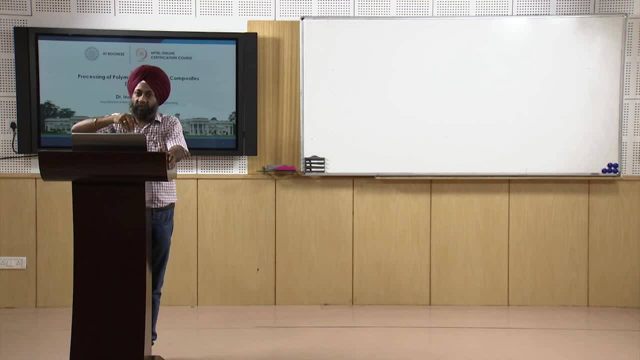 of pellets or granules is gravity fed from a top mounted hopper into the barrel of the extruder. i have already explained. the raw material is in a hopper. it is gravity fed means it comes down by its own weight. additives such as colorants and ultraviolet inhibitors. 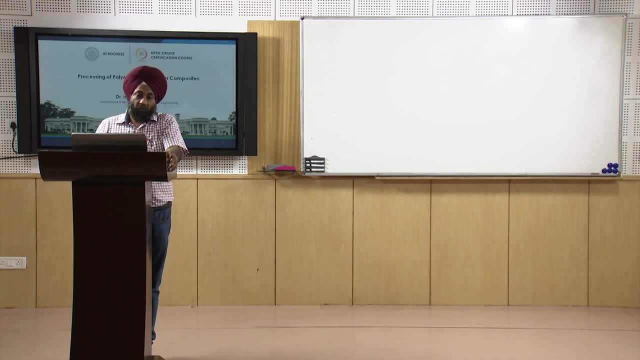 can be mixed in the hopper. now, this is important. you have seen so many different colors of products were there in the very first slide. there was yellow color, green color, black color. so we, these coloring agents, we have to adapt, add in the hopper. we have to prepare a batch of the raw material which will have the pellets. 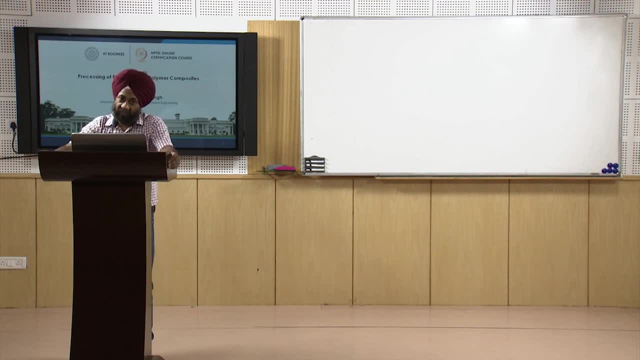 other additives, sometimes fire retardants, may also be added at the raw material mixing stage only. so here coloring agent will be added. similarly, ultraviolet inhibitors can be mixed in the hopper. now ultraviolet inhibitor. many a time we see decoloration of the plastic products takes place. if suppose the bucket lies in the sunlight everyday and for months. 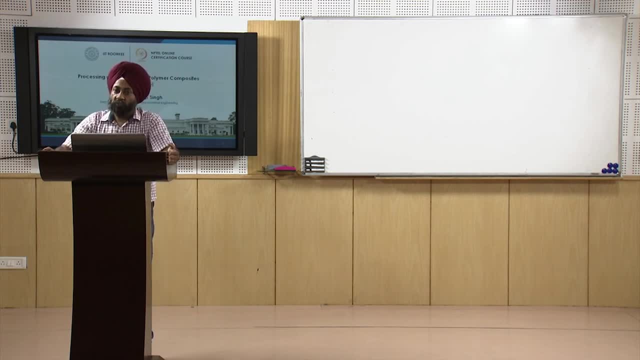 all together for years, all together the decoloration takes place. so we can add some inhibitors which inhibits the decoloration of the plastic parts, all those things- raw materials, can be added in the hopper. plastic materials enters through the feed throat and comes into contact with the rotating. 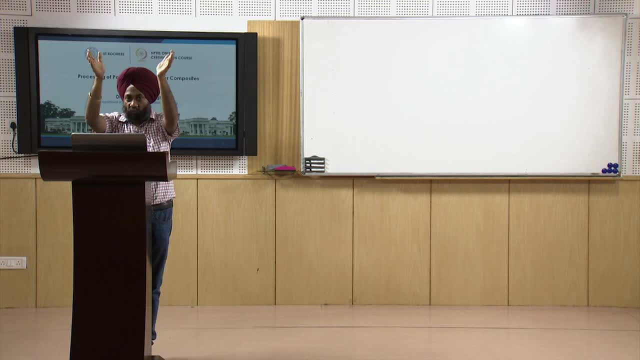 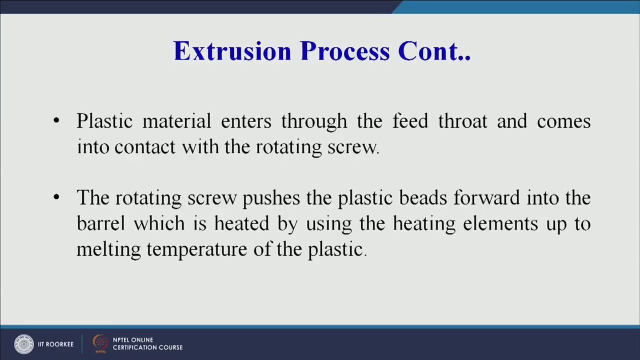 screw. now feed throat is at the end of the hopper. so you have a hopper, there is a feed throat at the end and through that the raw material in the form of pellets and other additives adds ah, enters into the barrel. the rotating screw pushes the plastic beads or plastic pellets forward. 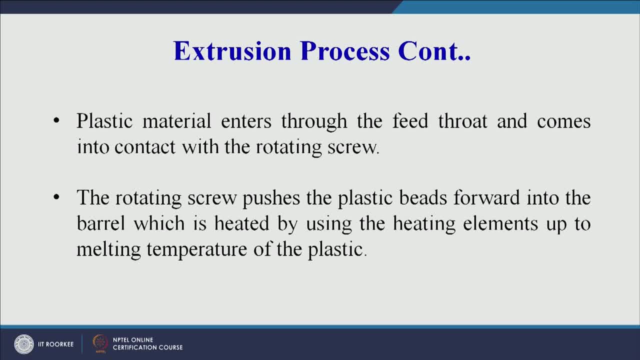 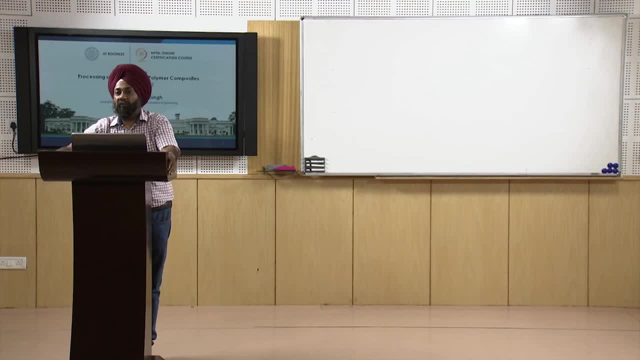 into the barrel, which is heated by using the heating elements up to the melting temperature of the plastic. so we will melt the plastic because of the heating arrangement that we have provided around the barrel. so once the plastic is in the molten state it will start to flow, and then we will push this molten plastic with the help of a rotating screw. 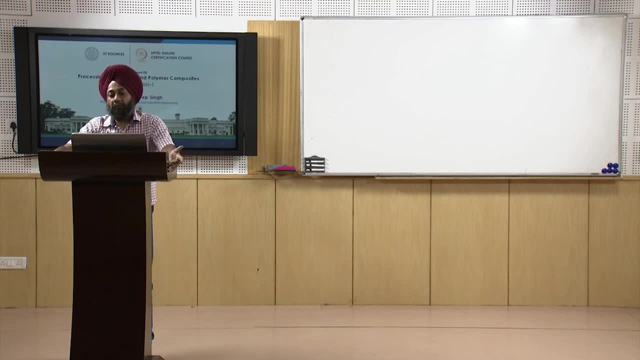 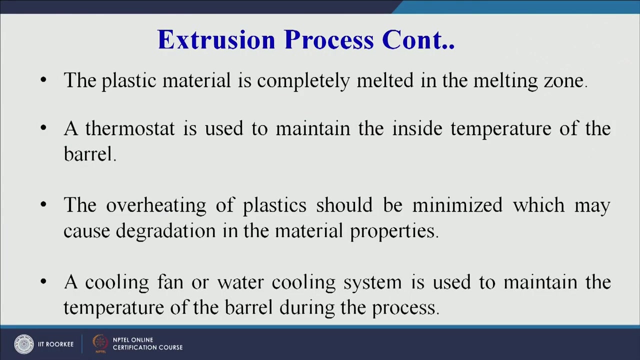 through the die. so the next stage is the die. the plastic material is completely melted in the melting zone. so we will see the design of the screw and there are three zones specifically for specific task that we will see later. so the plastic material completely melts in the melting zone. the thermostat is used to maintain. 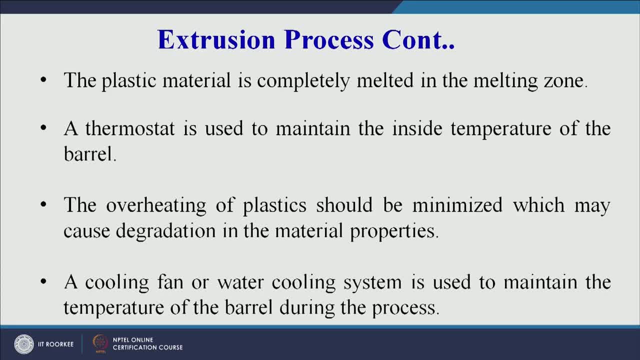 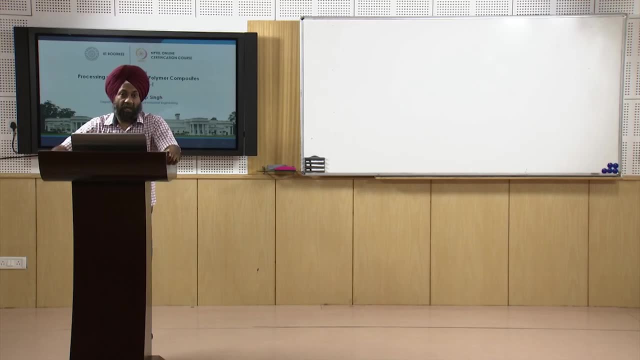 the inside temperature of the barrel because we need to maintain that temperature by the time we push our molten plastic through the die. the overheating of plastics must be minimized, which may cause degradation of the material properties. Now we have to see that how much temperature we should give to the plastic overheating. 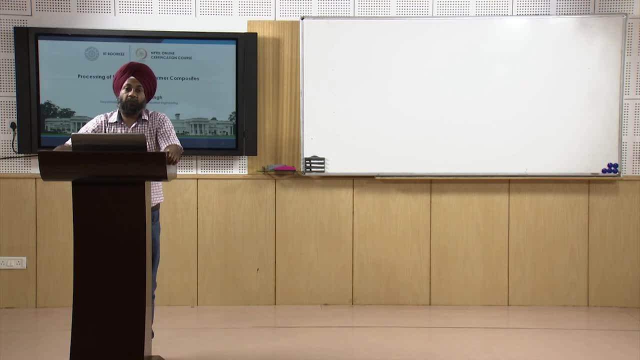 of the plastic is also not is also not advisable. why? because it will degrade the properties of the product that we are making. So we have to be judicious in the choice of the temperature that we are going to give to the heating elements, so that we are able to control the properties of the final product. 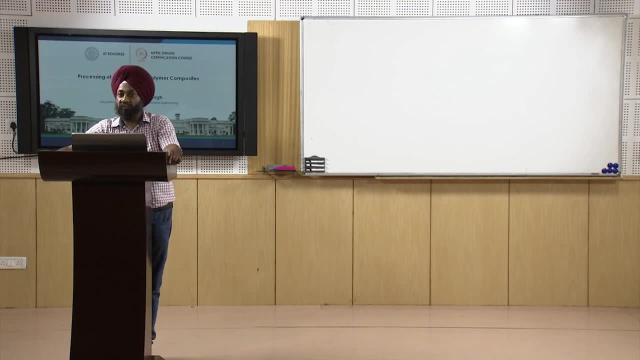 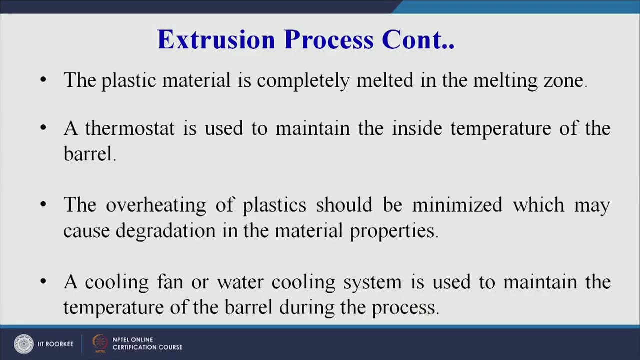 so the overheating of plastics has to be avoided. we should always keep this thing in mind. a cooling fan, So that is the water cooling system, is used to maintain the temperature of the barrel during the process. so this is an another important point: that we need to maintain the temperature. 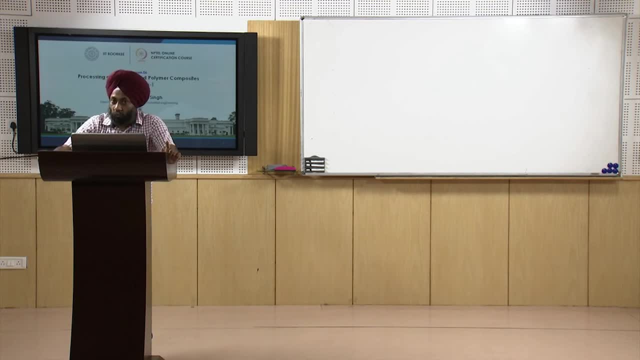 in the barrel. for that we have heating elements. in order to avoid the overheating, we have the cooling arrangement, that is, the fan or a cooling system is provided. Now there are other arrangements, as I have told you. the diagram that was shown is a very simplistic way to explain that. how. exclusion process. 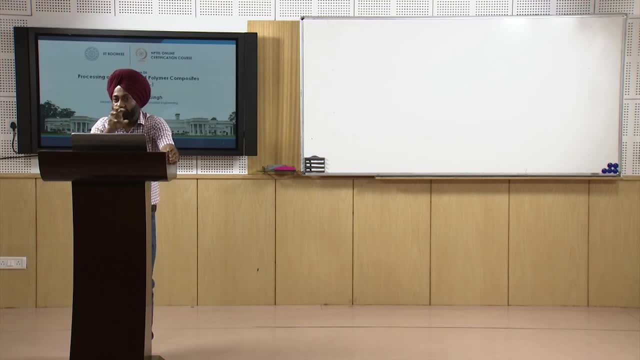 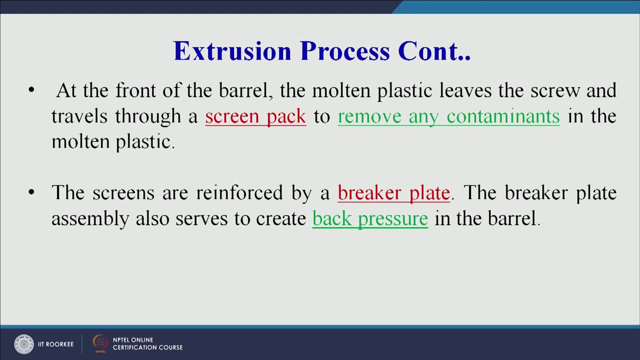 Actually works, but there are other arrangements also for specific tasks. so we have seen that over. for avoiding the overheating, we have to provide the cooling system. similarly, at the front of the barrel, the molten plastic leaves the screw and travels through a screen pack. Now what is the role of this screen pack? it, the role of screen pack, is to remove any contaminants. 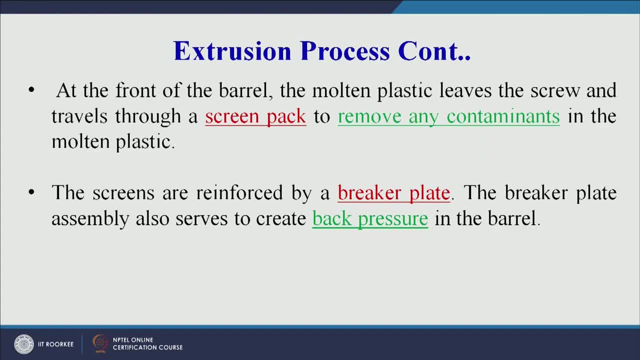 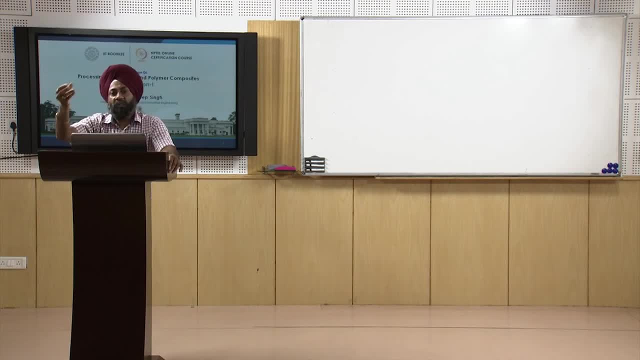 in the molten plastic. many a times we are using the plastic pellets. there may be some undue particles or non-wanted particles all mixed with the pellets. that may travel through the barrel, through the screw. they may be fed through the die. so we need to check that these. 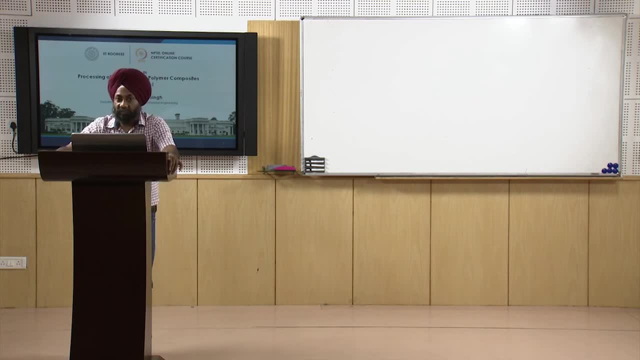 particle, they may be sometimes causing harm to the die. also, as I have told you, die is the most complicated part of the whole system and the shape, size, surface finish of the product depends upon the die. so if your die wears out very fast, the that is the most costly. 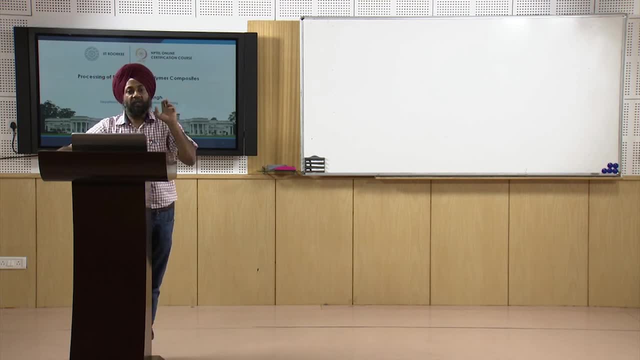 component. So therefore we do not want any additional or any undue particle going into the die. that has to be avoided, and for avoiding that we can put a screen pack which will only allow the plastic to go through into the die and will arrest all other particles which are 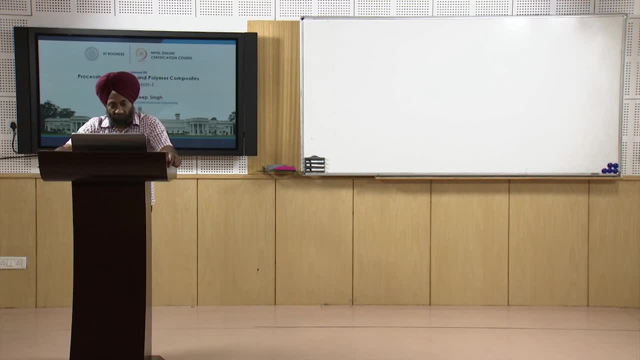 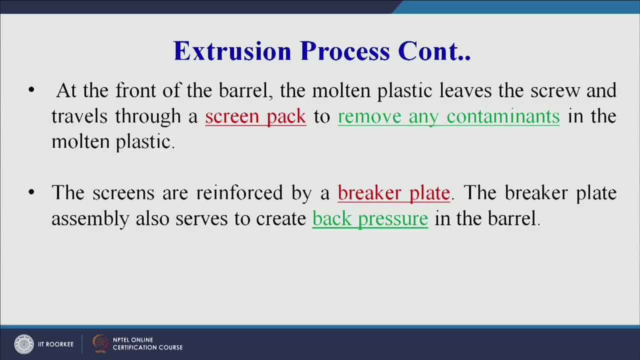 not required or unwanted particles or unwanted impurities. So the role of the screen pack is to remove any contaminants in the molten plastic. the screens are reinforced. Now what is the role of the breaker plate? the breaker plate assembly also serves to create back pressure in the barrel. now back pressure. why back pressure is required there? 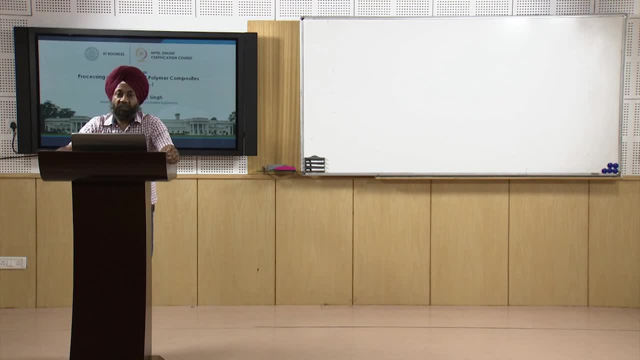 are two, three terms that have come up on this screen. one is screen pack. that is to avoid the flow of the undue or unwanted particles or impurities. with the molten plastic it will arrest those. secondly, the breaker plate. now breaker plate will apply. also help us in applying. 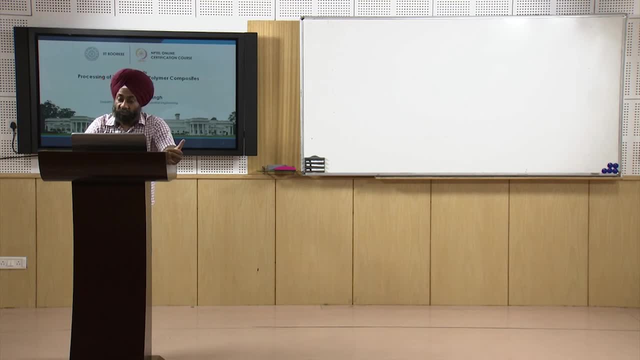 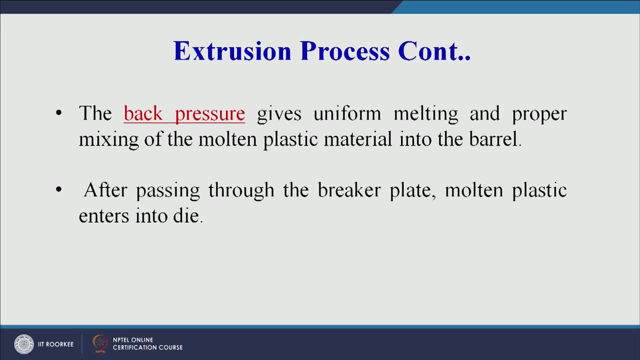 the back pressure. Now, what is back pressure? we will see why back pressure is required. the back pressure gives uniform melting and proper mixing of the molten plastic in the barrel, So that back pressure has to be maintained so that we are able to properly mix the plastic. 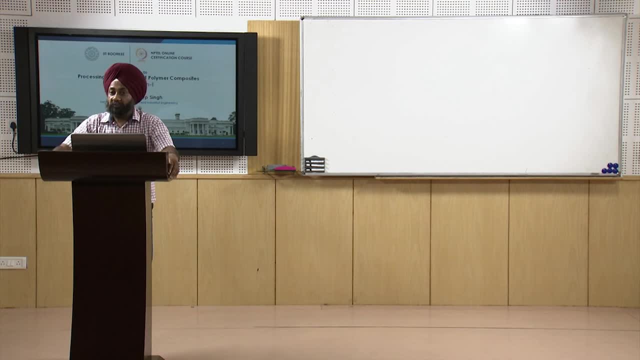 the all the pellets melt and there is proper mixing, as we, as I have already told that we may be adding some additional, we can say, additives in the hopper. so proper mixing is one of the purposes Of the barrel. then it is supported by the back pressure as well as the uniform mixing. 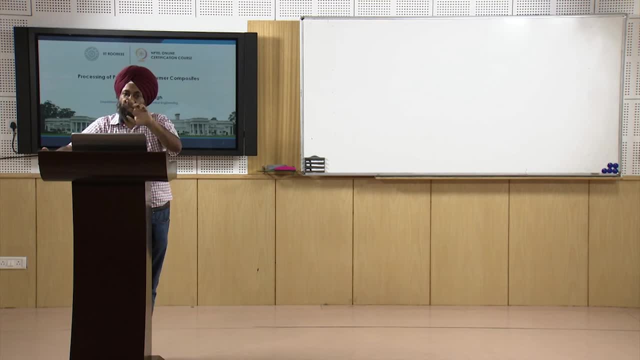 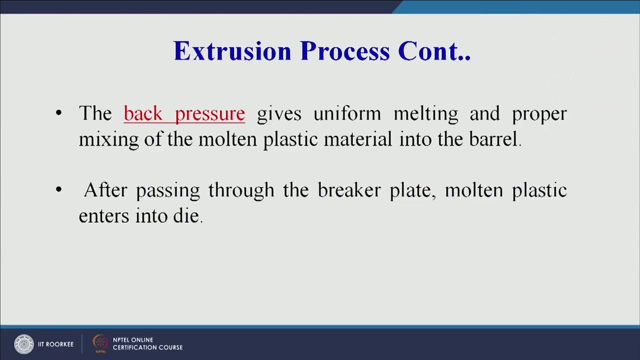 is one thing and uniform melting is the other thing. so both are m mixing and melting. so back pressure helps us to achieve these two m's. the two m's are mixing and melting, uniform melting and proper mixing. After passing through the breaker plate, the molten plastic enters into the die now die. 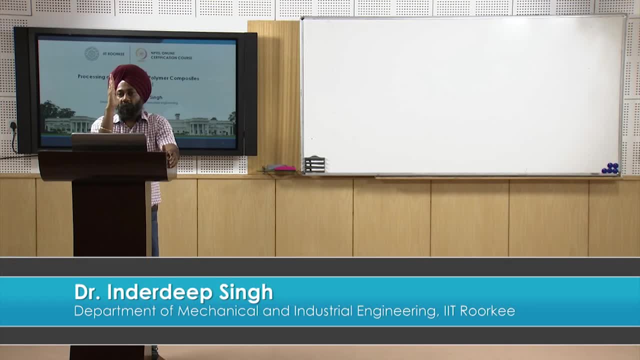 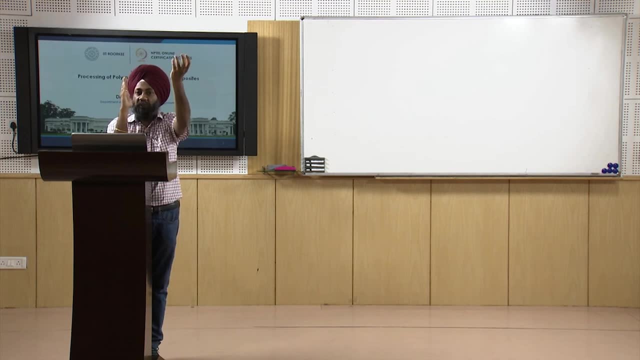 is, we can say, is one stage, Die is one stage. before that, what has happened? the molten, sorry, the polymer pellets or the plastic pellets have travelled from the hopper through the, we can say thot they have entered into the barrel. then there is a rotating screw, there is a heating arrangement, the heating. 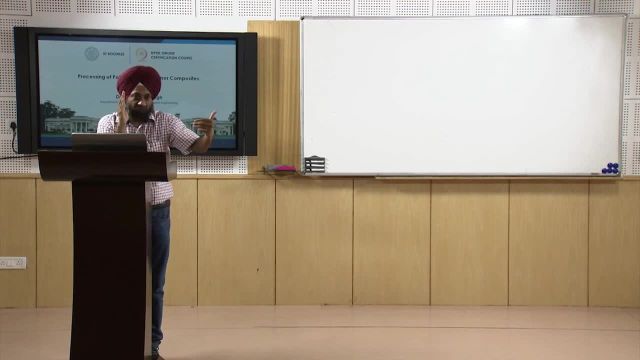 arrangement is heat providing heat to this plastic raw material. the material is getting melted. this melted material is pushed forward. 18. We have a type of a rotating screw and this screw also results in the mixing and melting of the raw material. there is a screen pack which avoids the undue or the unwanted particles. 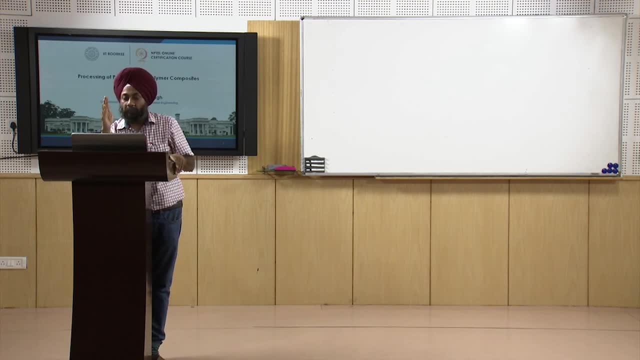 to move through, move along with the plastic, and then there is a breaker plate which provides the back pressure which ensures the proper mixing and proper melting of the polymer pellets. So this thing has already happened. now the material is entering into the die. and once the material enters into the die, 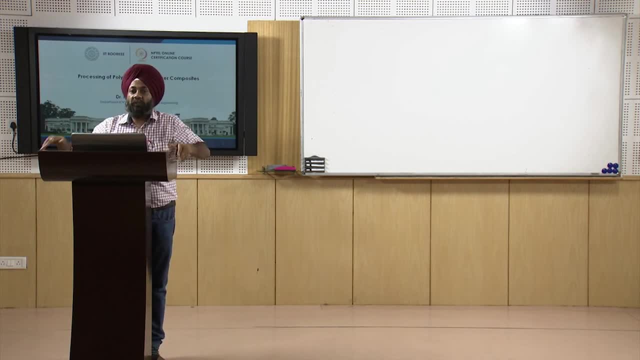 into the dye, it will take the shape. so, as per our principles of processing of polymer, three things are very, very important. first thing is heating. we have to heat the raw material. that has already happened till now. second is forming. that is giving shape to the raw material. so now the dye will help us in the second step, that is giving shape to the raw. 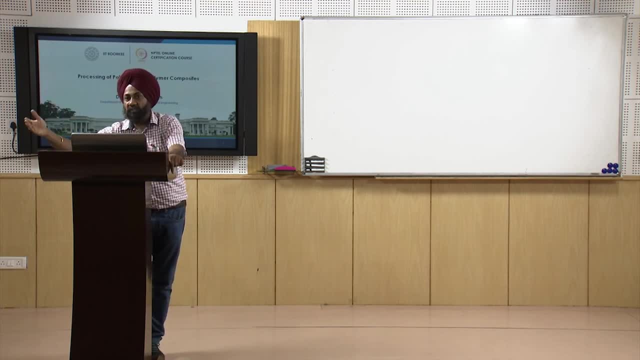 material. and third part is cooling. so cooling we will see later. now we have finished our stage one, that is, melting, mixing the raw material. now the raw material is ready to be deformed into the desired shape, and that will be achieved by the help of a dye. now the after passing. 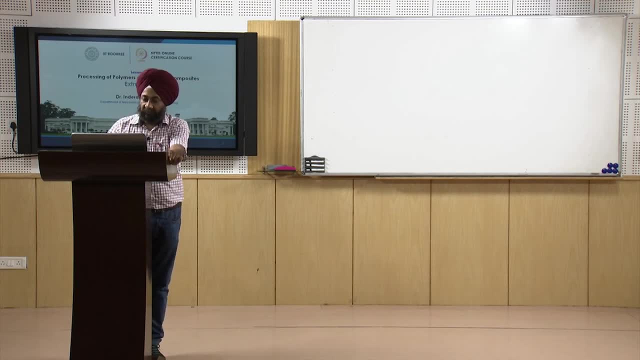 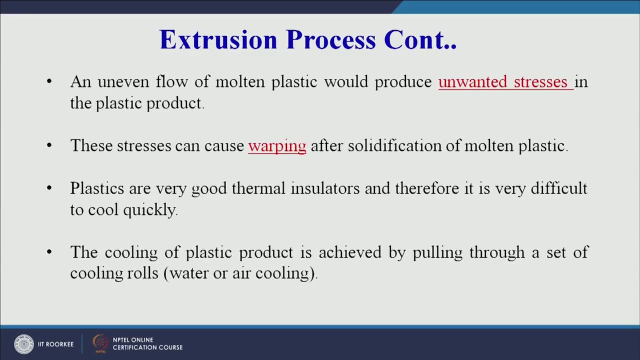 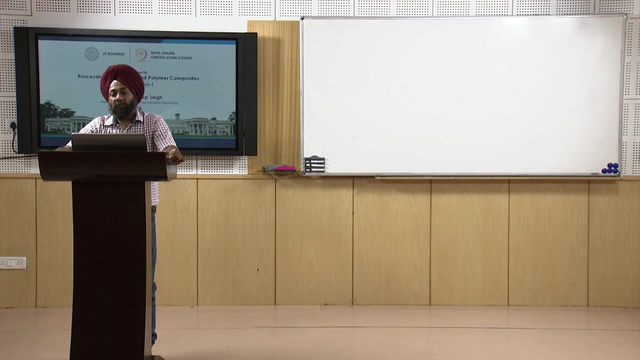 through the breaker plate, the molten plastic enters into the dye. now an uneven flow of the molten plastic would produce unwanted stresses in the plastic product. so we have to ensure that the plastic is not getting into the mold and the molding process is not done. so we have to ensure a uniform flow, or a even flow of the molten plastic through. 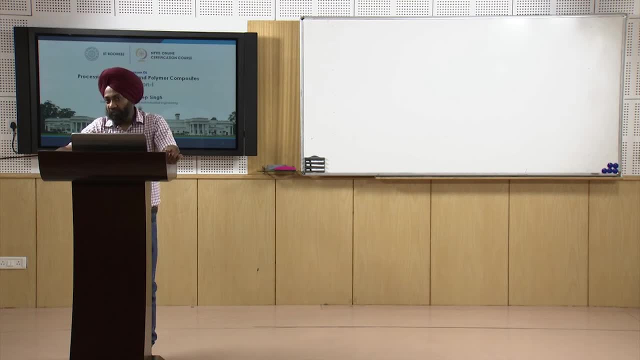 the dye. so why? because otherwise unwanted stresses will develop and unwanted stresses will cause warping after the solidification of the product. so this uniform flow of the molten plastic has to be ensured now. plastics are very good thermal insulators. they are not good conductors of heat and electricity and therefore it is very difficult to cool. 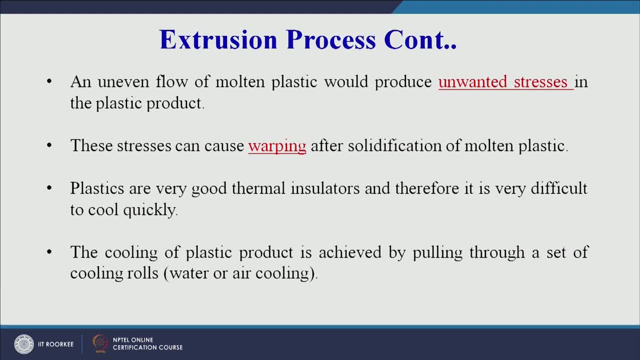 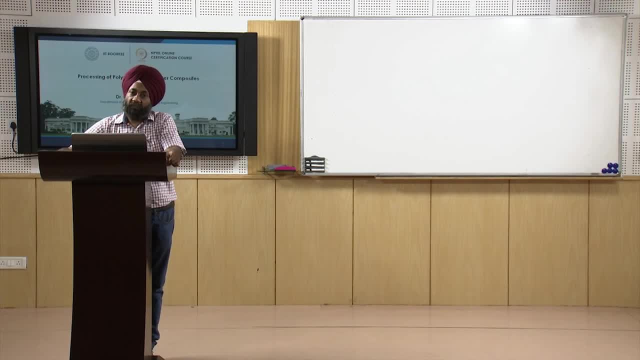 them quickly. so the cooling of the plastic product is achieved by pulling through a set of cooling rolls, as we have seen in our diagram, the. we can always supply water cooling or air cooling for making of gardeners pipe or horse pipes. the product, when it comes out from the dye it is fed through the water. there is adequate. 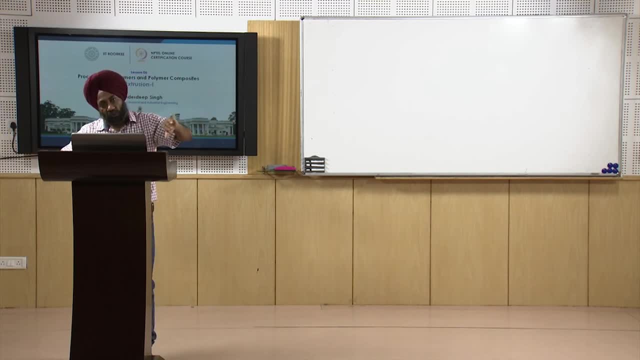 length of this water column or a water chamber through which the product is passed. and when it comes out of the water chamber or water channel it is solidified and it is in the final shape, or it is in the final shape In the useful shape, or useful. it become the useful product so cooling can be achieved. 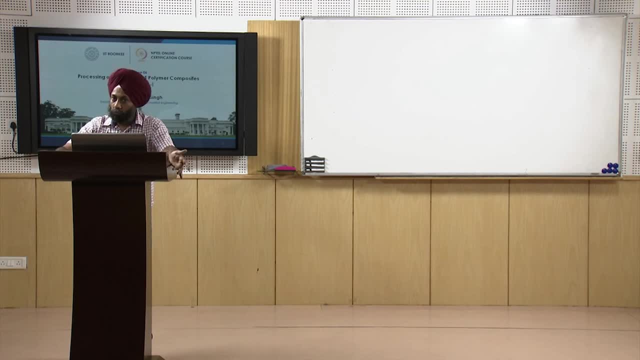 through water also. cooling can be achieved through air also. so 3 steps now have been completed: heating, melting of the plastic, deforming in the dye and finally cooling, whether it is air cooling or it is water cooling, and on the way there are 2, 3 things that we have. 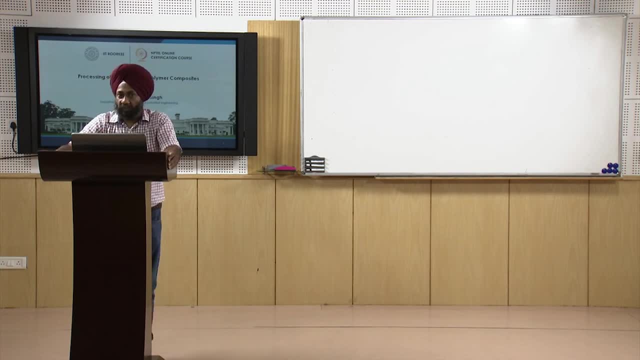 to ensure that no undue particles travel with the molten plastic. there is adequate mixing of the plastic So that we have added there is a uniform flow of the plastic through the dye as well as after it comes out of the dye. that has to be ensured. 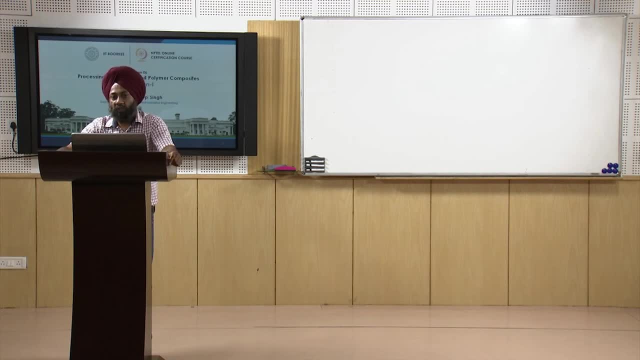 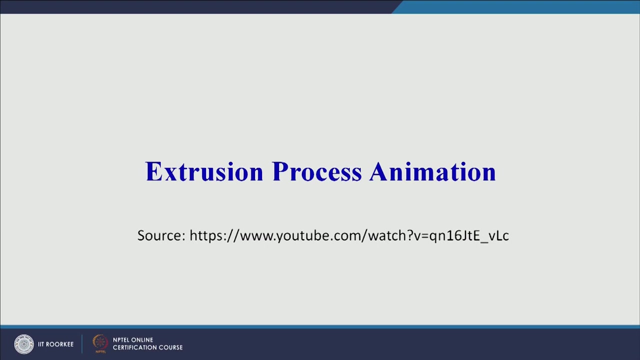 Now we will try to see a very simple simulation or animation. number of such animations are available on general platforms, general video platforms. one such platform is youtube. on youtube, number of such animations are available as open source. We have given the source also wwwyoutubecom, and this video is available, so you can see there are other videos also.